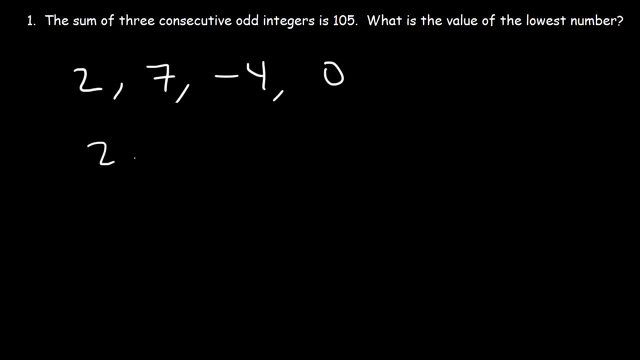 an even integer and an odd integer. So even numbers are like 2,, 4,, 6,, 8,, 10.. Odd integers are 3,, 5,, 7,, 9, and so forth, So consecutive odd integers. 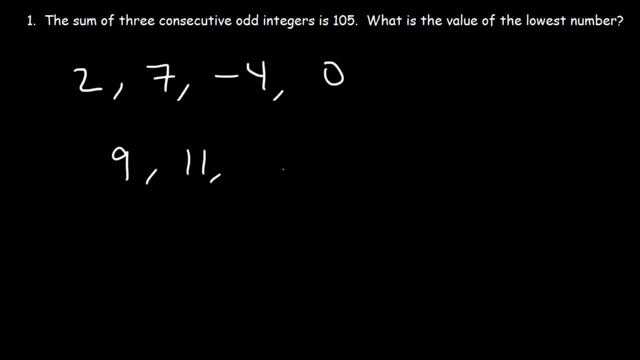 for example, would be like 9,, 11,, 13,, 15.. You would skip the even ones. So these are consecutive odd integers. 5,, 6,, 7, 8 are simply consecutive integers. 12,, 14,, 16,, 18, that's a list that represents consecutive even integers. So make sure you. 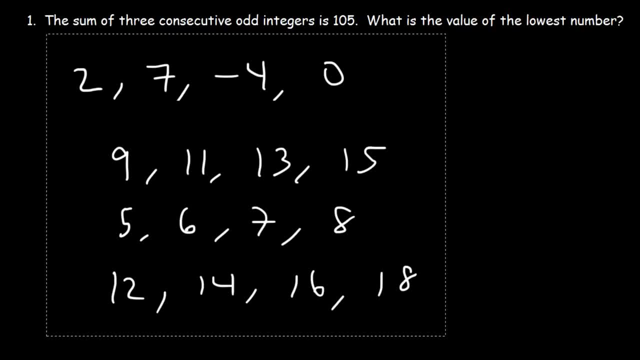 understand the difference. So, looking at this problem, the sum of three consecutive odd integers is 105.. What is the value of the lowest number? The quick and simple way to get the answer is to take 105 and divide it by the number of integers in the list, which is 3.. 105 divided. 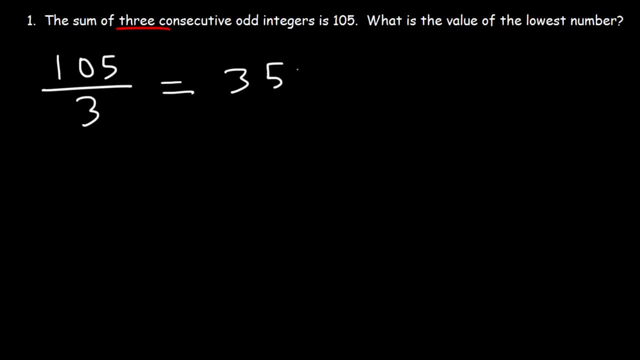 by 3 is 35, and 35 is an odd integer. This number will give you the average or the middle number of the list. If that's the middle number, then the other two numbers are 33 and 37.. 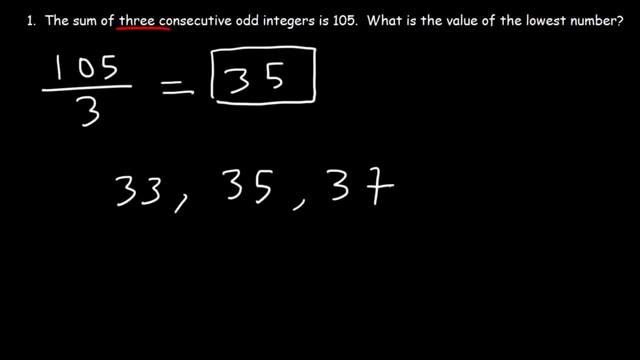 So these are three consecutive odd integers that add up to 105.. And you can type it in your calculator: 33 plus 35 plus 37 is indeed 105. So those are the three numbers. Now we're looking for the value of the lowest number. The lowest number is 33.. 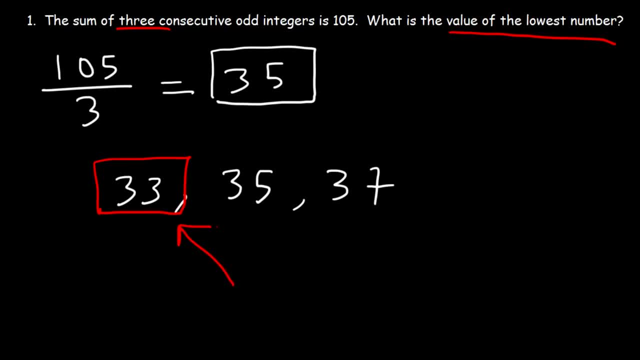 So that is the answer. So that's how you can find the answer, the quick way. But let's say, if you have to show your work, What can we do? The first integer we're going to call x. The second integer is going to be x plus 2.. 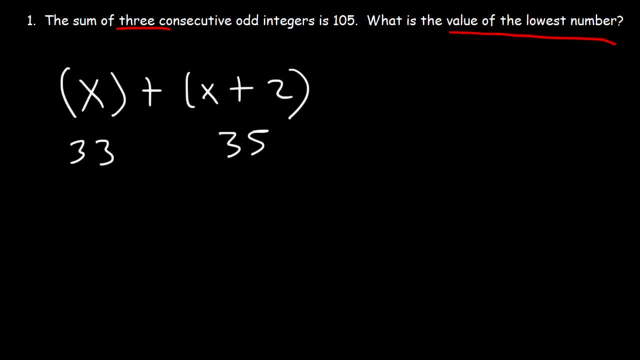 So if 33 is x, 35 will be the next one. 33 plus 2 is 35.. The third integer is going to be x plus 4.. And these three integers have to add up to 105.. So now let's combine like terms: x plus x plus x is 3x. 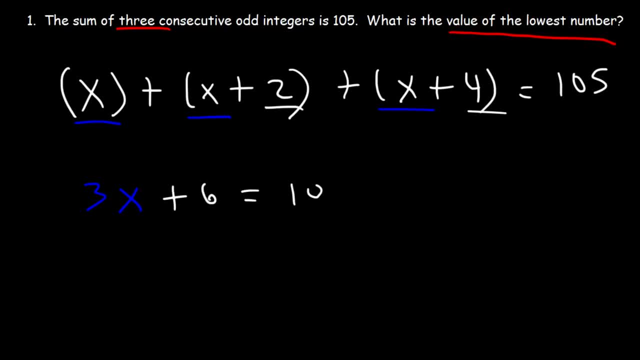 2 plus 4 is 6, and that's equal to 105.. Now let's subtract both sides by 6.. 105 minus 6 is 99.. And 99 divided by 3 is 33.. So therefore, the first number is 33.. 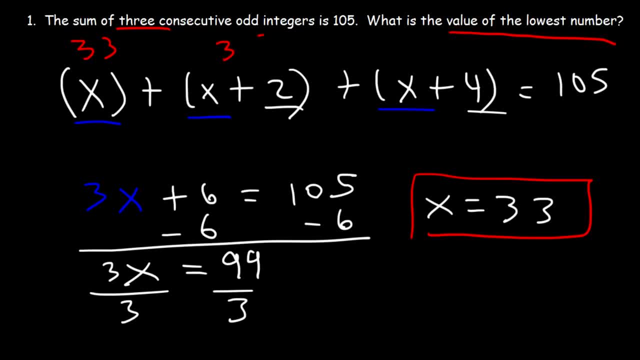 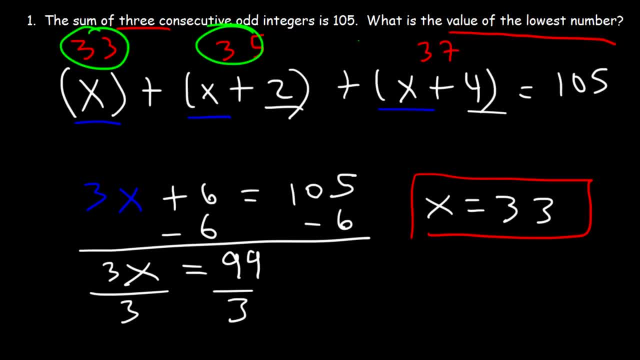 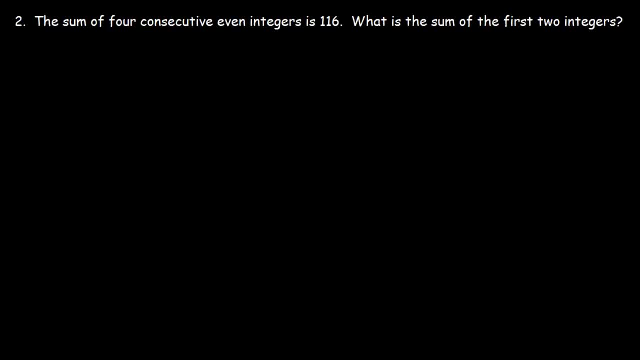 And that's how you can show your work. That's how you can get all three numbers. So 33 is the answer. Here's another example: The sum of four consecutive, even integers is 116.. What is the sum of the first two integers? 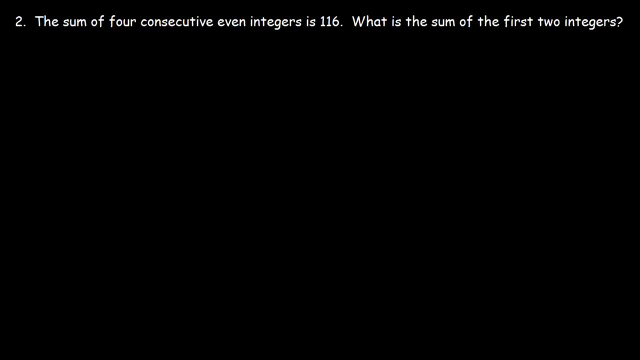 Well, first let's find the four even integers. So what we're going to do is find the average of the four numbers. 116 divided by 4 is equal to 29.. So 29 is the average And 29 is not an even number. 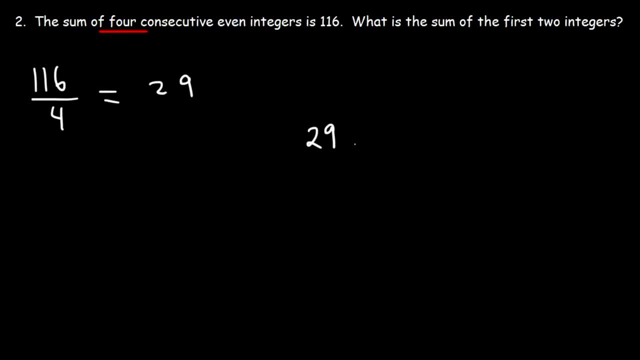 So 29 is not in the list. However, 29 should be the middle number If there's four numbers. that means two numbers should be to the left of 29, and two numbers should be to the right of it, Meaning two numbers. we have two even numbers that are greater than 29,. 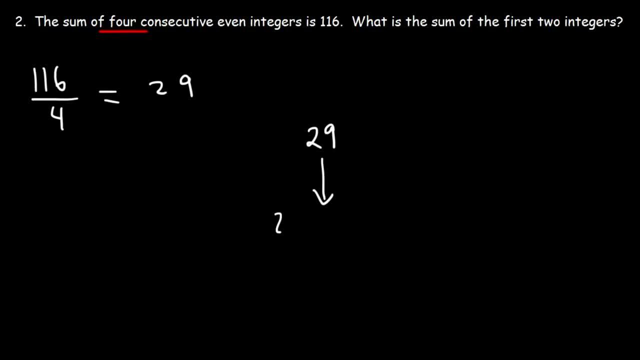 and two even numbers that are less than 29.. So it's going to be 28,- 30.. 29 is right in between 28 and 30, and also 32 and 26.. If you average 28 and 30, you get 29.. 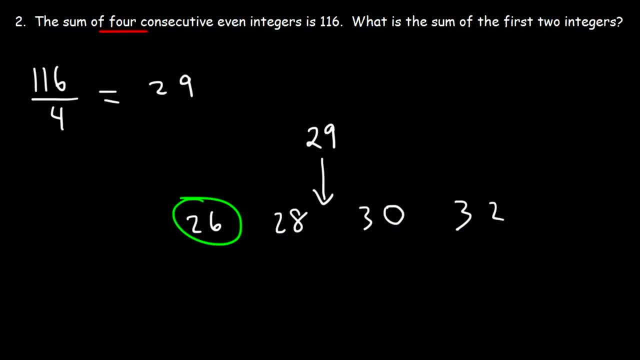 If you average 26 and 32,, you get 29.. So these are the four consecutive even integers And if you add up these four values- 26 plus 28, plus 30, plus 32, is equal to 116.. 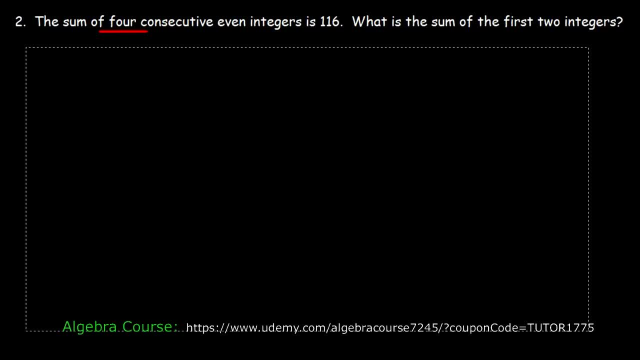 Now let's show our work to get these answers. The first integer we're going to call x. The second integer is x plus 2.. The third integer is x plus 4.. Even numbers differ by 2.. And the fourth is going to be x plus 6.. 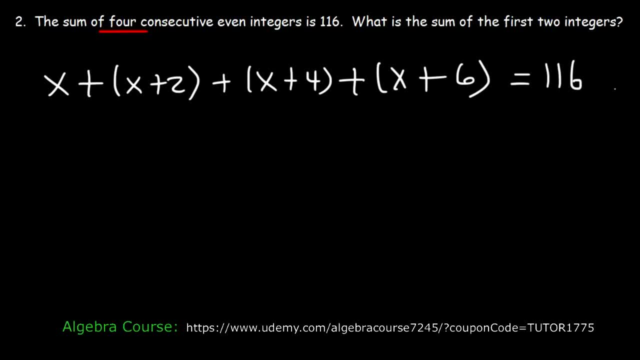 These four numbers have to add up to 116.. So let's go ahead and find the value of x, x plus x plus x plus x is equal to 4x. 4 plus 6 is 10, plus 2,, that's 12.. 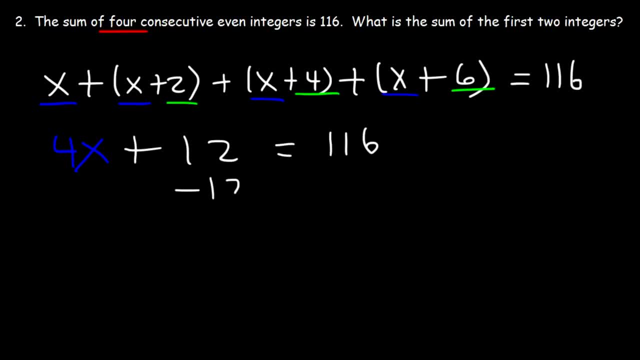 So 4x plus 12 is equal to 116.. 116 minus 12 is 104.. And if we divide both sides by 4,, 104 divided by 4 is 26.. So the first number is 26.. So if x is 26,, x plus 2 has to be 28.. 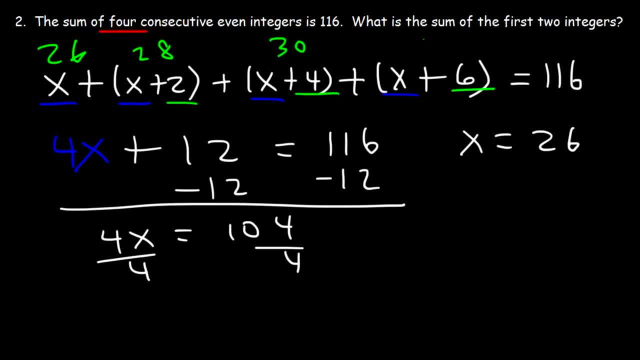 26 plus 4 is 30, and 26 plus 6 is 32.. So these are the four numbers. Now the question wanted the value of the sum of the first two integers. The first two integers are 26 and 28.. 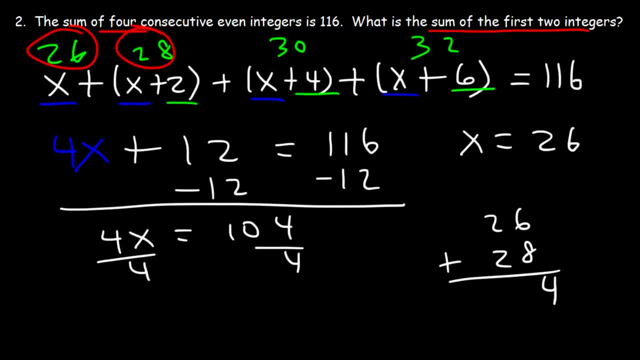 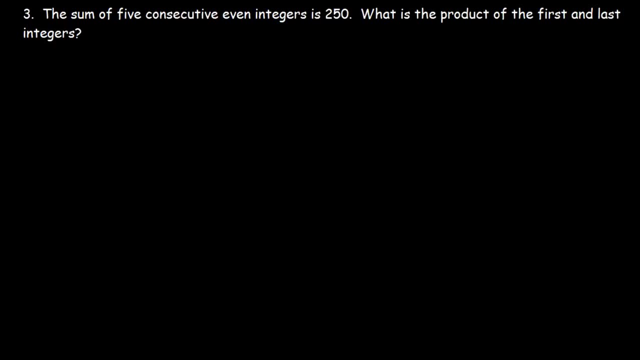 So we got to add these two numbers: 8 plus 6 is 14.. 2 plus 2 plus 1 is 5.. So the sum is 54.. This is the final answer, Number 3.. The sum of five consecutive even integers is 250.. 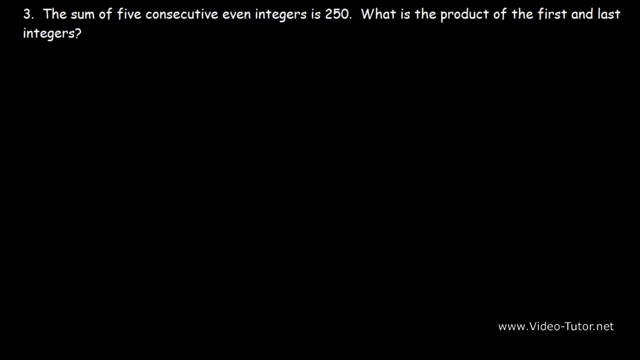 What is the product of the first and last integers. So let's find the average. The sum is 250, and there are five numbers, So let's divide it by 5.. 250 divided by 5 is 50. So this is going to be the middle number out of the five numbers, because this number is even. 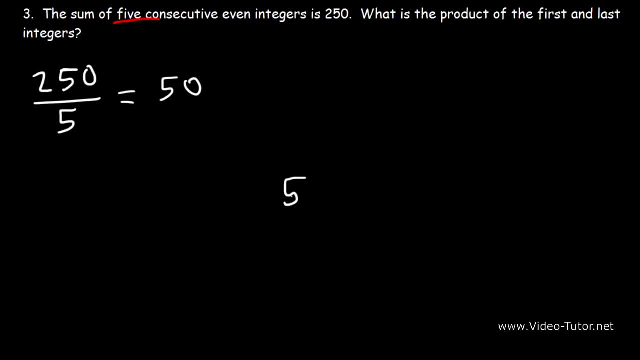 So it's going to be included in the list. So 50 is the middle number. There are two even numbers that are less than 50. So that's going to be 48 and 46.. Now there's two even numbers to the right of 50, or greater than 50.. 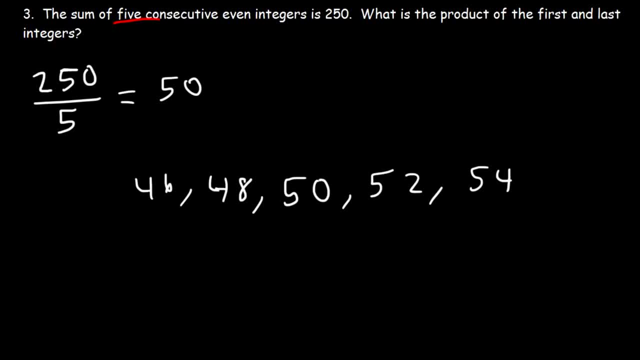 That's 52 and 54.. So these are the five consecutive even integers And if you look here, you'll see that there are two even numbers And if you add up the five values, this will give you 250.. Now our goal is to find the product of the first and the last integer. 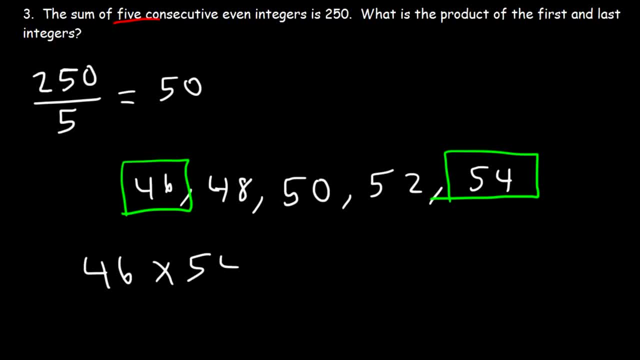 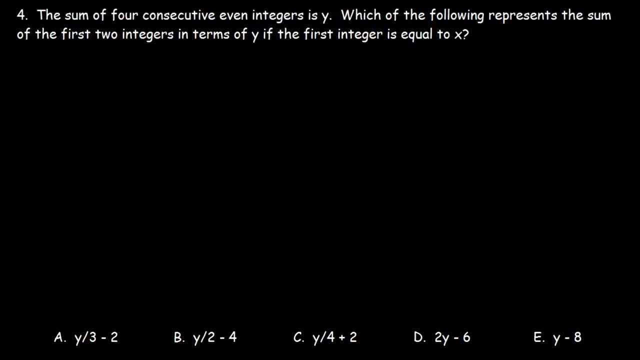 So we've got to multiply 46 by 54.. 46 times 54 is 2,484.. So this is the final answer, Number 4.. The sum of four consecutive even integers is 50.. The sum of four consecutive even integers is y. 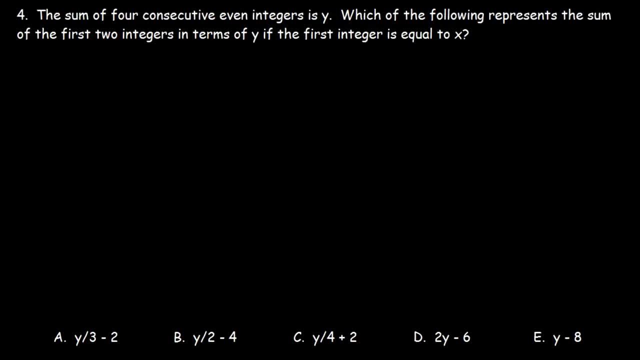 Which of the following represents the sum of the first two integers in terms of y, if the first integer is equal to x. So the first integer is x, The second integer is going to be x plus 2, because we're dealing with consecutive even. 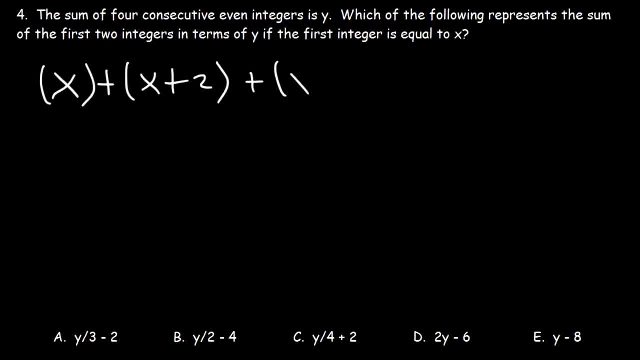 integers which differ by 2.. The third is going to be x plus 4.. And the fourth is going to be x plus 6.. And the sum is equal to y. So what do we need to do here? We need to find the value of x in terms of y. 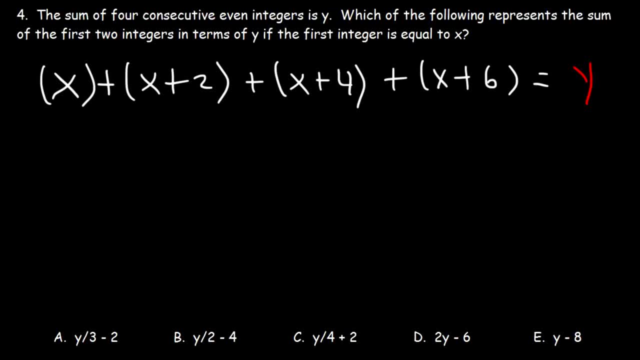 And then we could find the sum of the first two terms in terms of y, x plus x plus x plus x. we know that's going to be 4x. 6 plus 4 is 10, plus 2,, that's 12.. 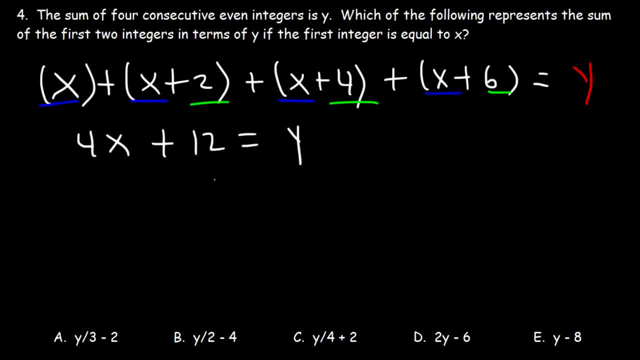 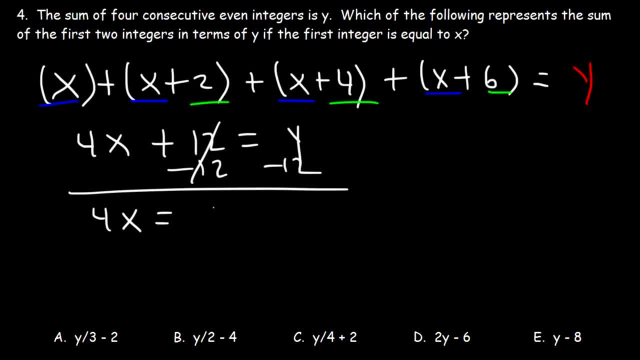 we can see that 4x is y minus 12. and now let's divide everything by 4, but let's do it separately. so x is equal to 1. fourth, y minus 3. 12 divided by 4 is 3. so this gives us the value of the first integer in terms of y.